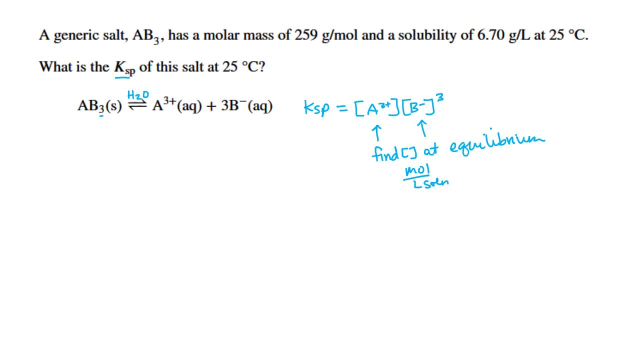 liters of solution and moles of B minus over liters of solution. So now the way that I would go about doing this is: it says this generic salt has a molar mass and a solubility. Okay, so this solubility right here tells me how much is going to dissolve in water. 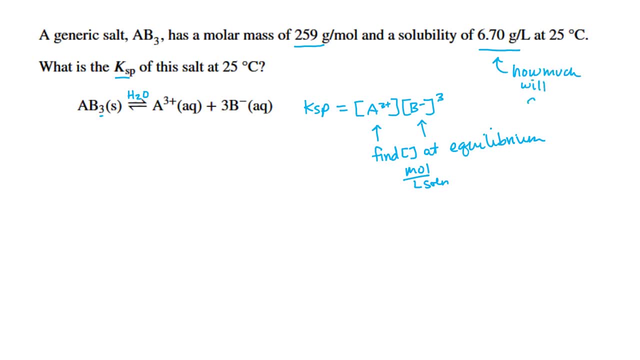 Okay. so because this tells me how much is going to dissolve, I can figure out what the molarity is of AB3 using the molar mass. So first step is find the molarity of AB3 using the solubility and the molar mass and then Waltenmaier at the количество of- believe it or not- the molarity. is 56 percent of the solubility. so moiety divided by molecular mass of AB6 and regular mass of AB6, and then you get this. So here is this same small rate calledMan global conversion rate. Now remember that concentration is going to be equal to the concentration at equilibrium. 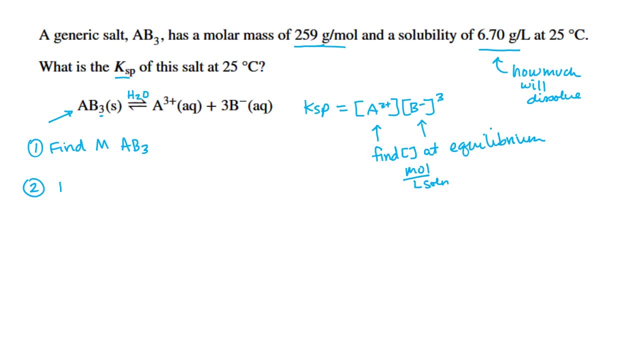 mass. Next, I'm going to use that to find the concentration of A3 plus and to find the concentration of B minus, Okay. And then the third step is I'm going to find KSP- Okay, And I'm going to use this equation right there to do that, Okay. So, first up, find the 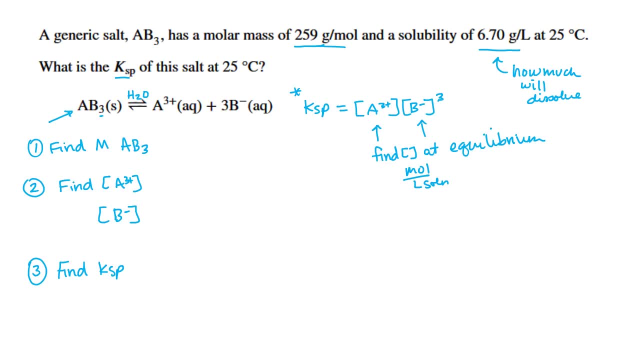 find the molarity or the concentration of AB3 using those numbers Okay. So if I have a solubility of 6.70 grams of AB3 over liters of solution, okay, and we can think of that as one liter of solution. Next we're going to use the molar mass. 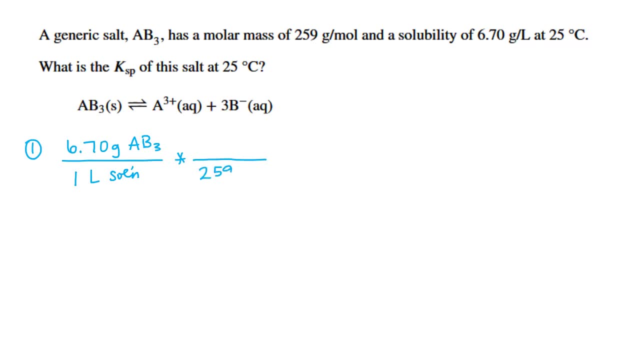 I have grams at the top, 7 grams at the bottom, So this is 259 grams of AB3 over one mole of AB3.. Okay, So my grams. I'm going to cancel with my grams and I'm left with moles per liter And the answer I get is 0.0258. 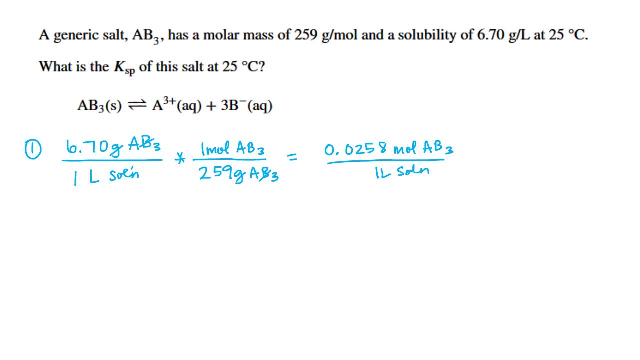 Moles of AB3 divided by one liter of solution. Okay, So there's my first step. My second step is: I'm going to use this number here to find the concentration of A3 plus right, And that's going to be moles of A3 plus over liters of solution. 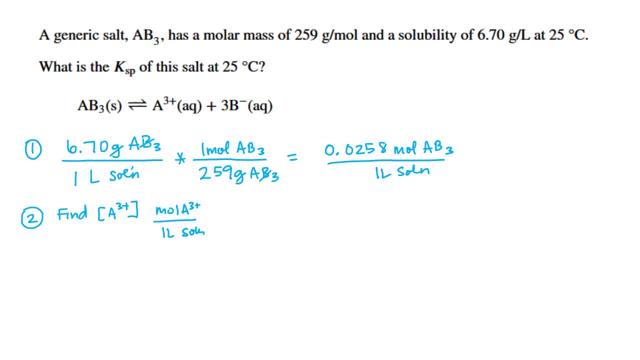 Okay. So to do that, I'm going to use the balanced equation And I'm actually just going to go from. we'll go with purple, I'm going to go from this number right here. So if I look at the balanced chemical equation, I have one mole of AB3 equals one mole. 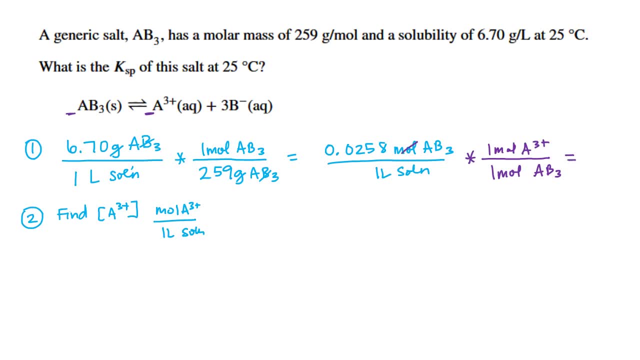 of A3 plus. Okay, Moles of AB3 are going to cancel, and I'm left with moles of A3 plus, and so this number right here equals 0.0258 A3 plus divided by one liter of solution. Okay, next step, Step number three, is to. 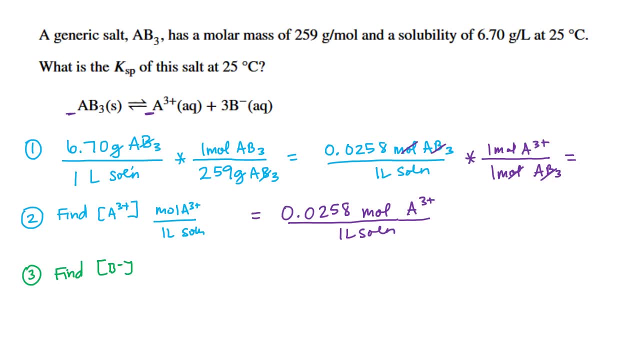 find the concentration of B minus Okay. so to do that, I can either start right here with moles of A plus or I can start with moles of AB3, so since this is here, we'll just start with this one, Okay. so what I'm going to do here is I'm going 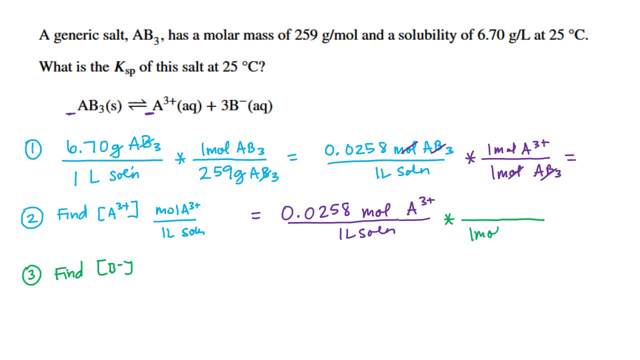 to take A3 plus. I know one mole of A3 plus equals three moles of B minus Moles of A3 plus. cancel and and I get 0.0258 times three moles gives me 0.0774 moles of B minus divided by liters of solution. 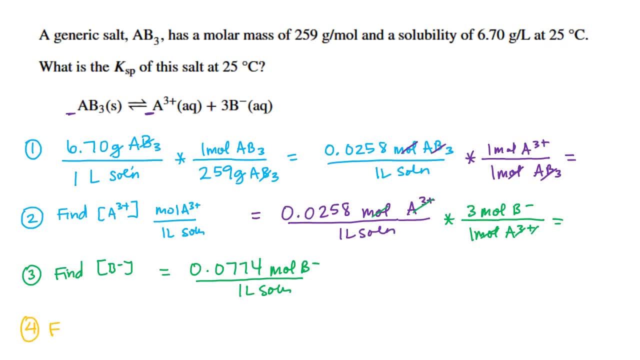 Okay, my last step, number four, is to find the KSP. Okay, so KSP is going to equal the concentration of A3 plus times the concentration of B minus to the third. So if we look back through our numbers, this number right here is the concentration of A3 plus.